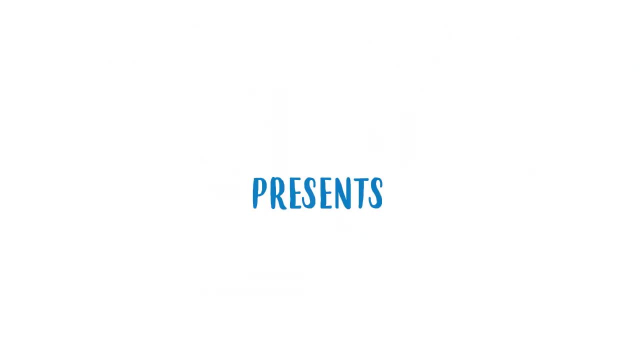 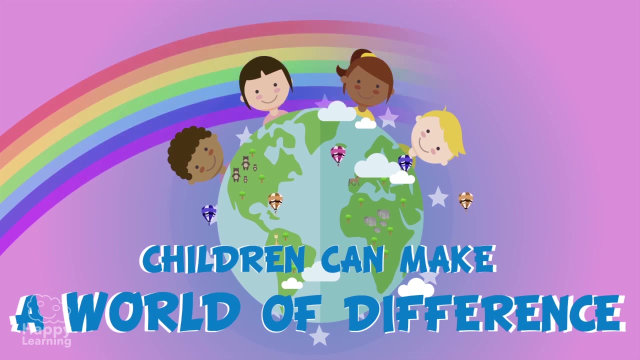 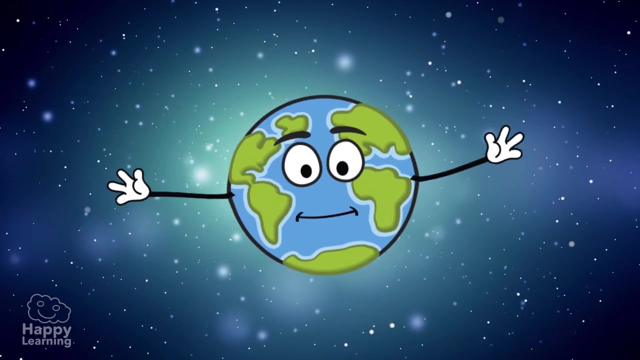 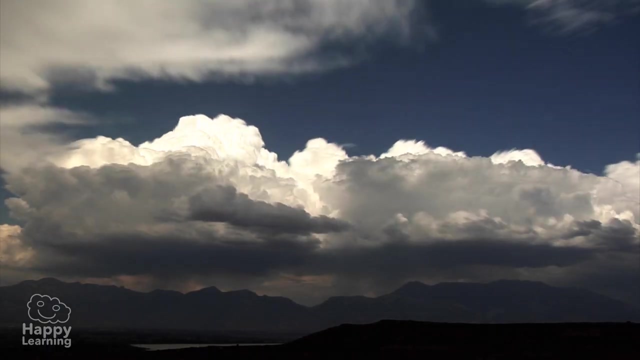 Hello, do you know who I am? I'm the Earth, Yes, the very same planet you live on, And I want to talk to you about a few things that concern me and that should concern you too. Everybody talks about what the weather is like or what it will be like if it's colder. 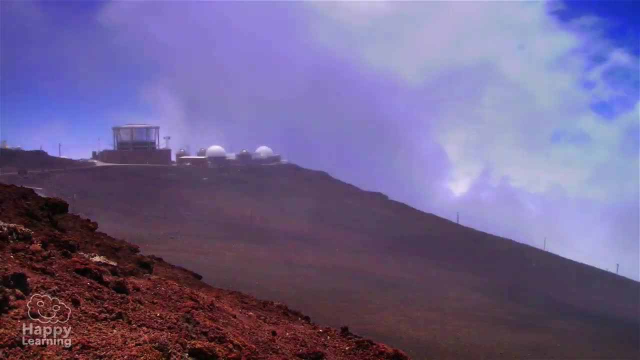 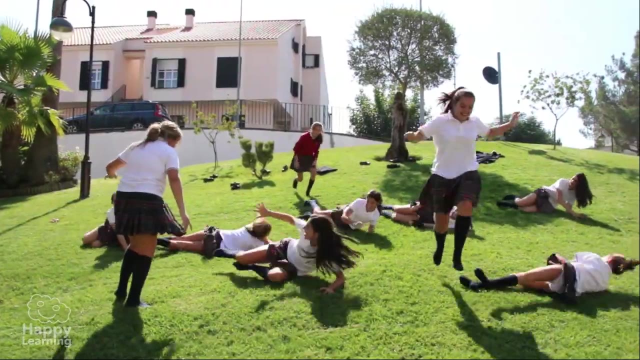 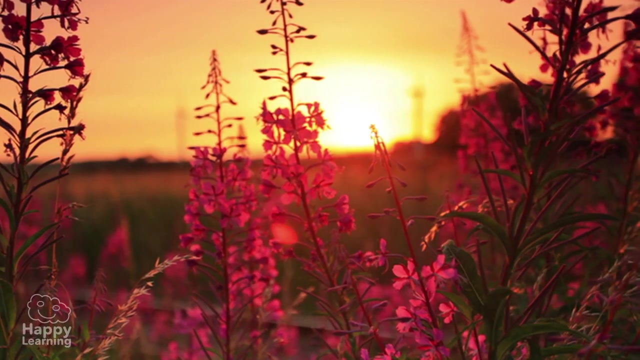 today than it was yesterday. if tomorrow it's going to rain, It's normal, because the climate is super important for our lives. It influences, for example, what we wear to school or if we can go and play outside, And it also affects all living things on Earth, including plants. 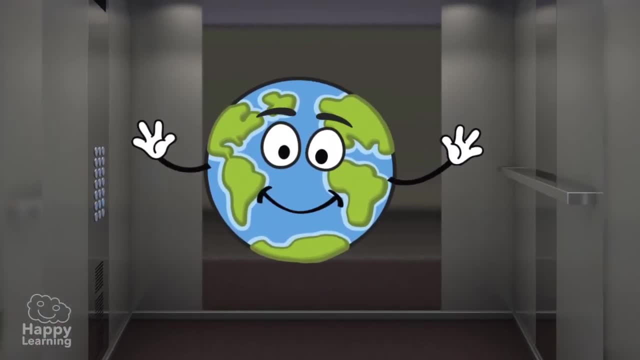 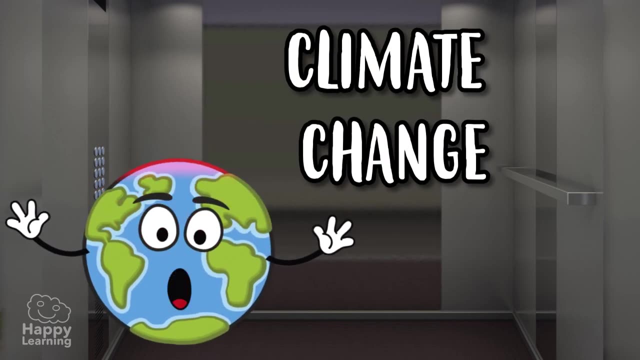 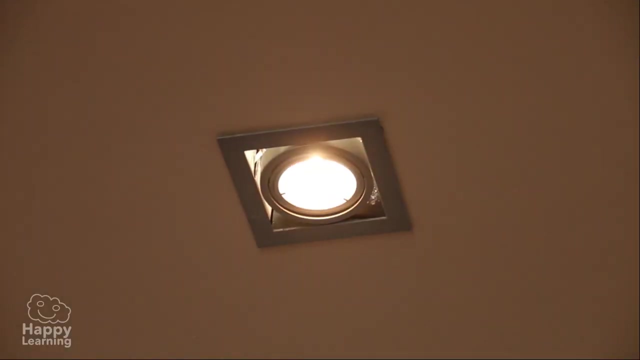 If you met me in a lift, do you know what? I'd tell you? That I am hot, very hot, which is due to climate change, which, as human beings, is something you are quite responsible for. Every time you turn on a light, the computer, the microwave, 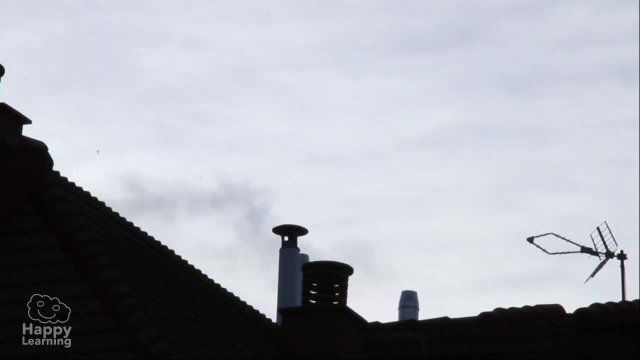 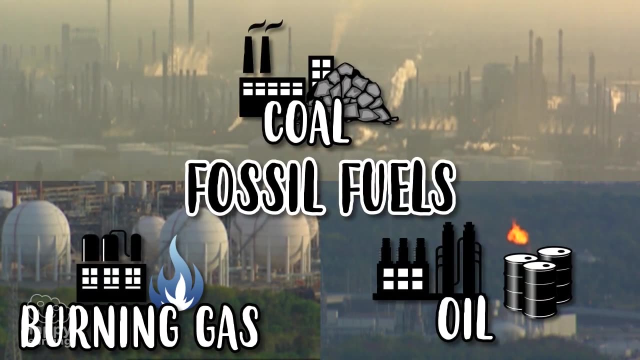 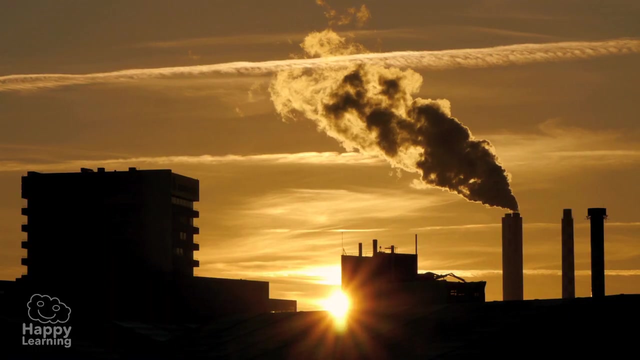 or every time you have a shower, you consume energy. This energy is mostly produced by burning gas, coal or oil, the so-called fossil fuels. When you burn them, you release gas into my atmosphere- tons and tons and tons of gas. 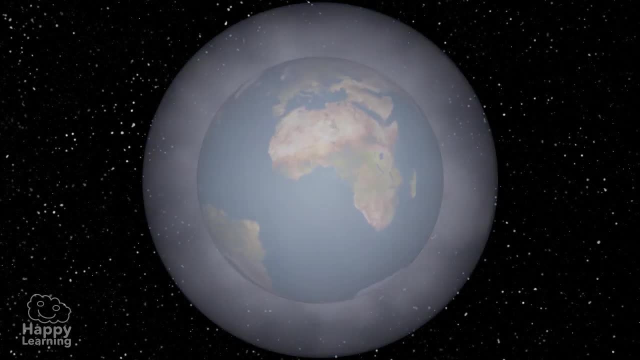 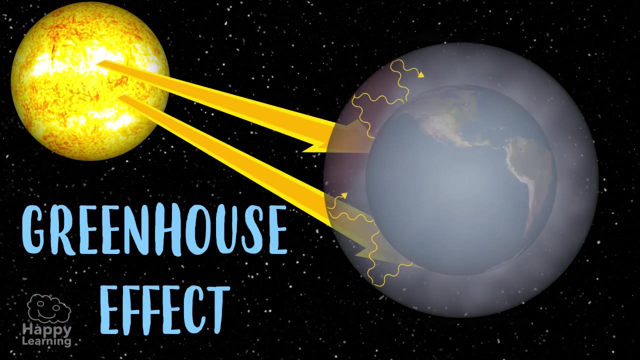 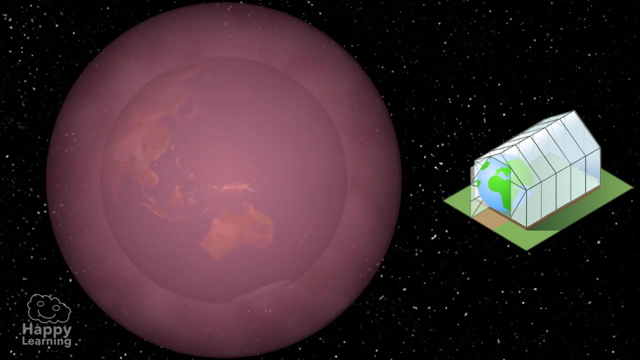 These gases stay in the atmosphere, forming a kind of ugly and dirty roof that retains heat. This is what is known as the greenhouse effect, because, like in greenhouses where plants are grown, this roof prevents heat from escaping, which makes me hotter and hotter. 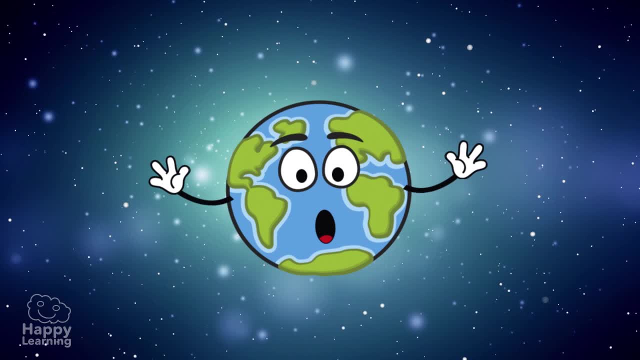 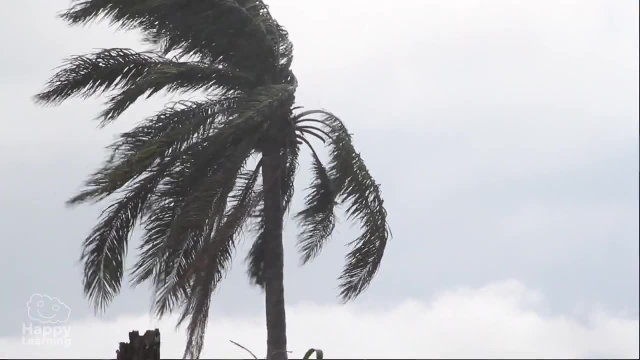 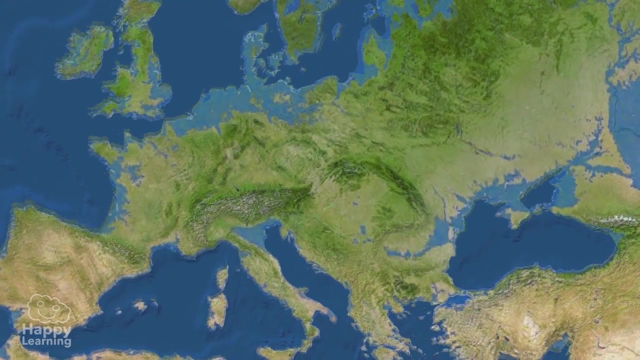 If this temperature rise continues, there will be very bad consequences for me and all living beings. It will cause severe storms and terrible floods. It will melt the ice at the poles, causing sea levels to rise until they flood coastal cities, Forest fires and 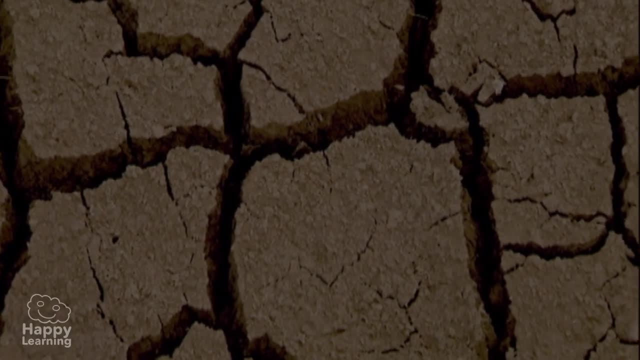 droughts will increase, turning formerly thriving areas into deserts. It would condemn entire species of animals that are inредate in the wild and do not менya have inredy in this land. It will miracles final comes alive. universal Design.